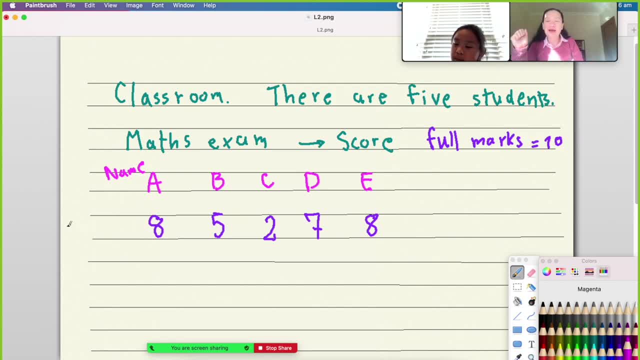 okay, um, it's a make sense. huh, you have five students and all of them have different score. the first student name, a, have eight from ten. we have five from ten. c, c has two from ten and d has seven from ten and e has eight. okay, what we going to do from here? 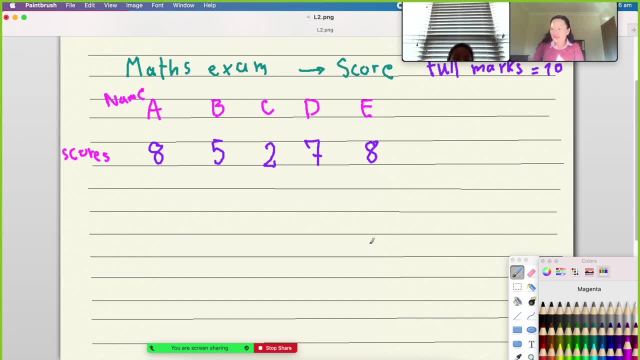 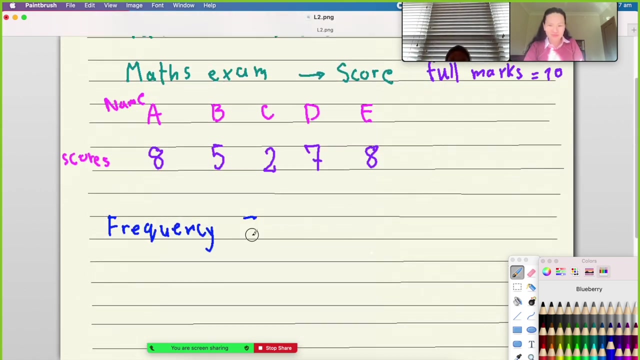 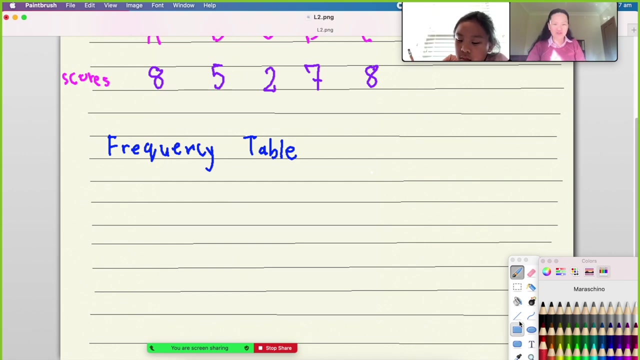 we try to write down is called frequency table. okay, okay, my grace, write down. okay, let's write it down: frequency table. oh, i, oh, okay, all good, frequency table. but we know from here, we would like, we would like to write up how you write our frequency table, the first row. it's going to be look like this. it look like a. 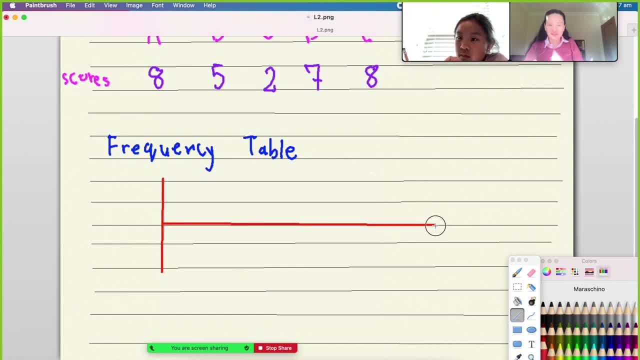 betsegal from b to b. only have a betsegal. we have to set a betsegal and frequency. that's the goتي switches, okay, okay, let's just look at this right here: here they're score, betel bean, they have score and frequency okay. 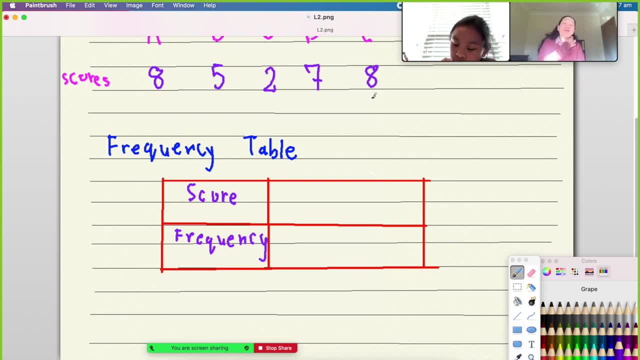 right down here scale. this one is score and this one is hit frequency. and he's going to frequency where how many score we have, we have to do, do. but before I do that one, how about we arrange them properly? first, from the minimum to maximum. what is the first one? huh? 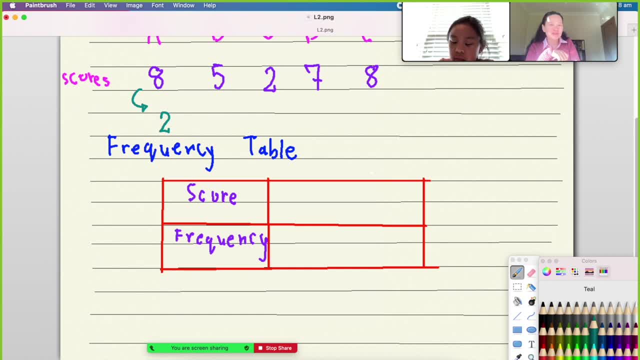 arrange them to you, mm-hmm. and then five, very good, then seven, seven and then eight, and another one, the last one, eight as well. yeah, we just rearrange them for minimum to maximum, for minimum to maximum to maximum: two, five, seven, eight, eight. okay, from here I know that they have one. 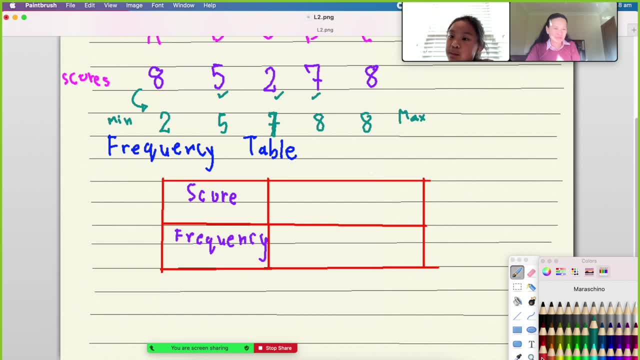 two, three, four. that fourth score in here, which is we have to call to, I write out to here, we have to call to, we write out to here, and frequency like a how many student who have to call to one one very good car? excellent, that it's really good because you're able to. 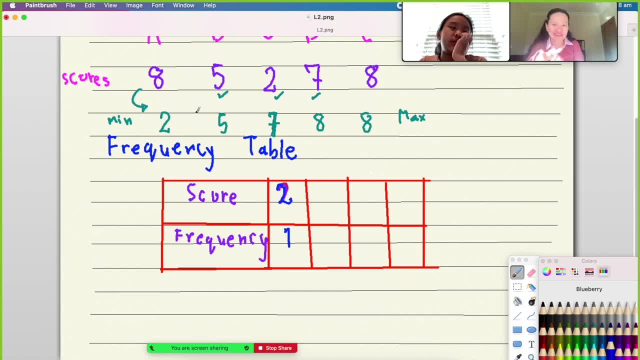 answer my question and you're able to analyze the data. okay, next score is five. what is the next score? eight and eight, eight, seven. yes, seven and eight. how many students have to call five? what one? how many students have to call seven- seven? how many students have to call five one? how many students have to call seven? 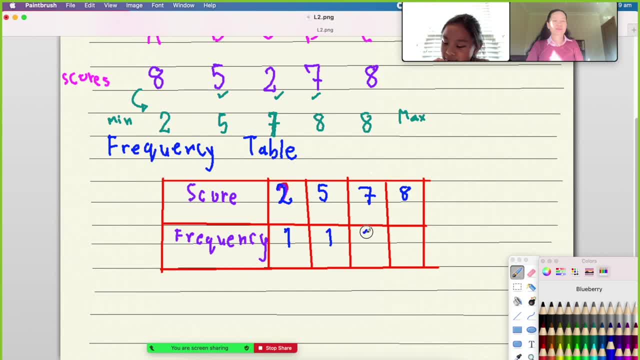 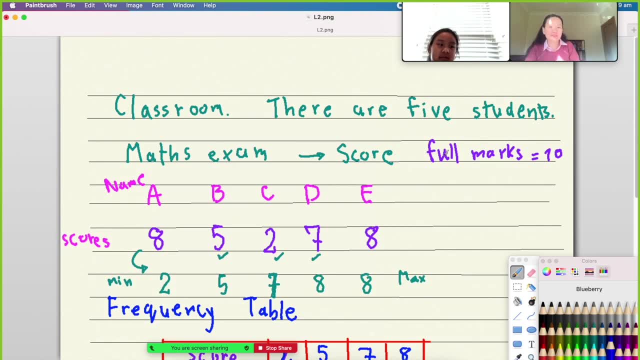 seven. how many students have to call seven? one, and how about to go eight, two. you one, and how about to go eight, two. you know that one, five students. so that mean the know that one, five students. so that mean the total number. total number, all right, total number equal of five. total number of student. 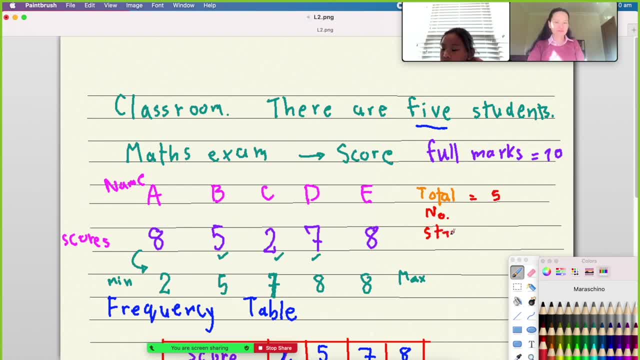 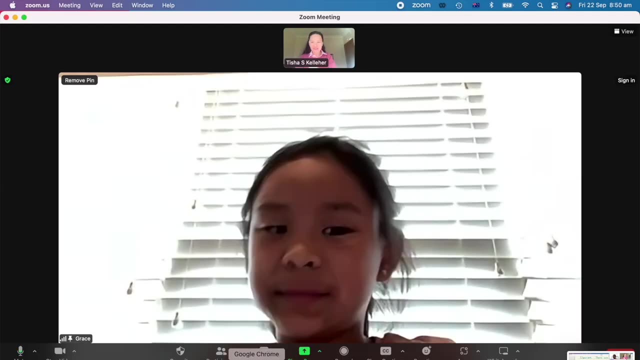 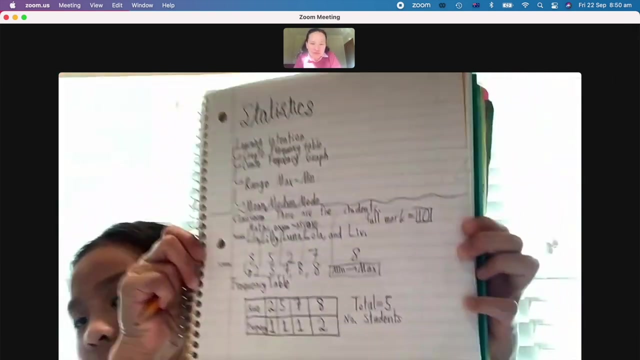 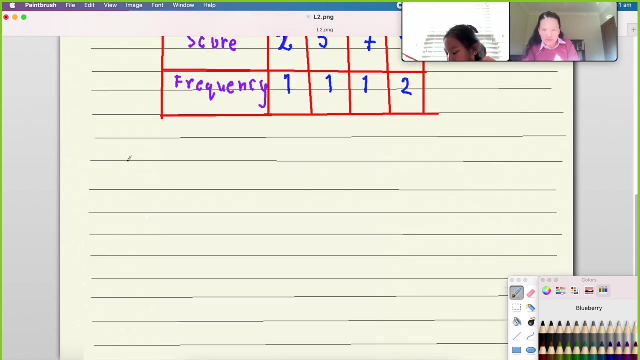 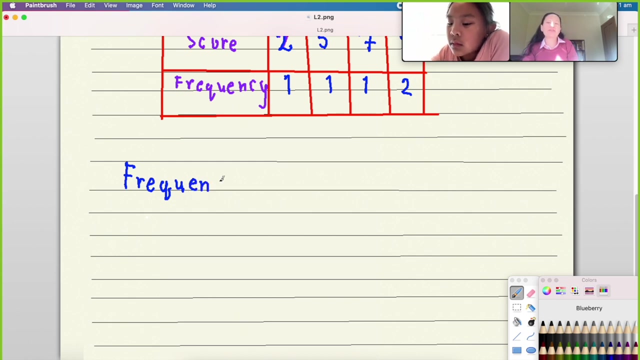 total number of students equal five. okay, good, can you see something? we have frequency table. I would like to see your note. huh, did you write down? well, now let's go next to frequency graph. you write down with me, please, frequency graph. well, you think it's easier for you if I write down on the paper that have line yes, so you prefer. 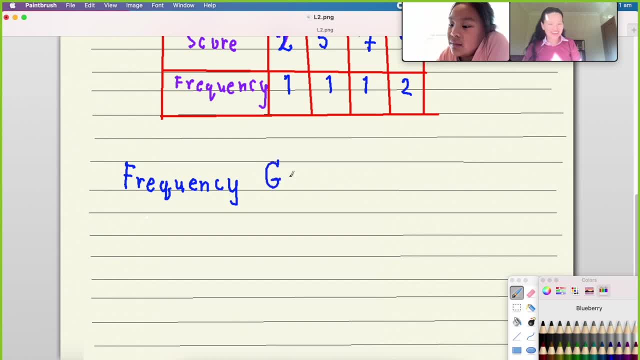 line. you know frequency graph. frequency graph: it's look a little bit different from other graph that we learn, because when we write down their exits Y and exit X, it is going to be like a compare between the score and the frequency. okay, now let's go to the next one. 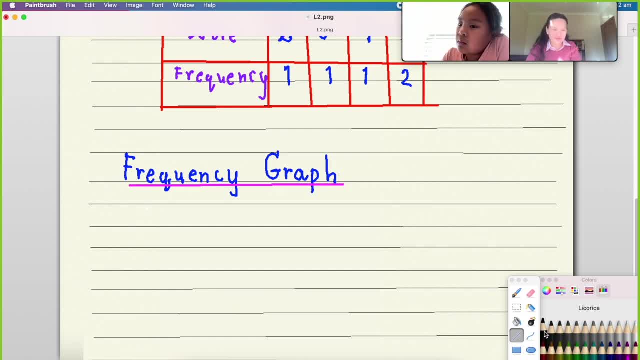 okay, now let's go to the next one. okay, now let's go to the next one. let you eat here. huh, oh my god, I can't let you eat here. huh, oh my god, I can't let you eat here. huh, oh my god, I can't believe that we able to make it exactly. 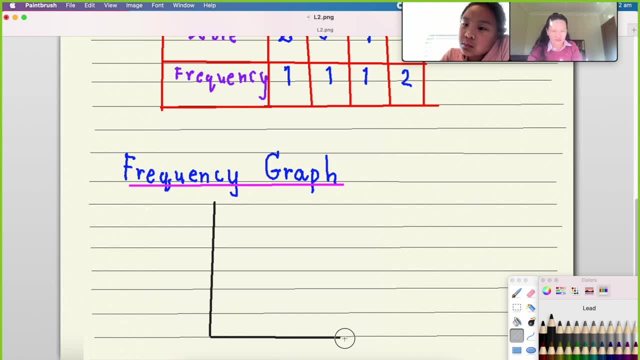 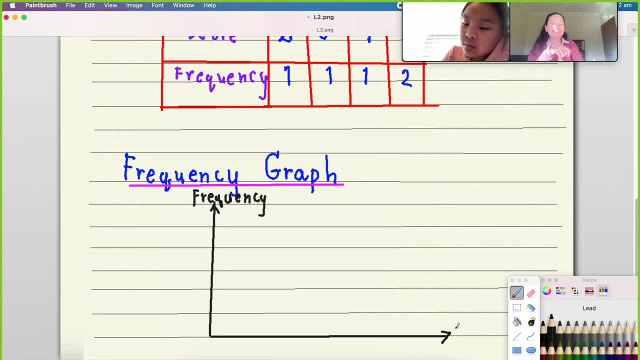 why, and this one is X. why? why it's it is frequency. why- and this one is X? why? why it's it is frequency x? exit is score. okay, next one. huh, come back here, it's different. great, you remember normally the graph. if we say seven, okay, seven is here, but 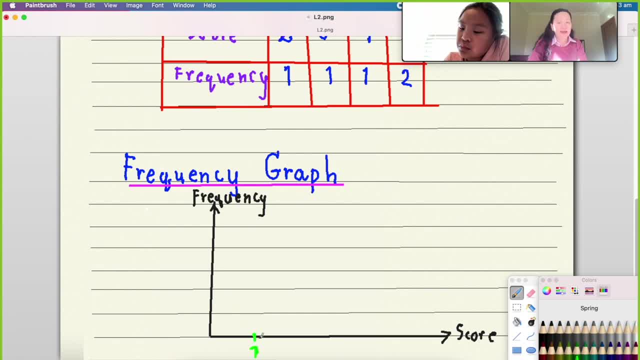 like on this small line, but in this case the graph, the score, going to be look like this: we have two, five, seven, eight. okay, let's see how about this. one is the score one, but because it's frequency graph again, when you write down one, you need to. 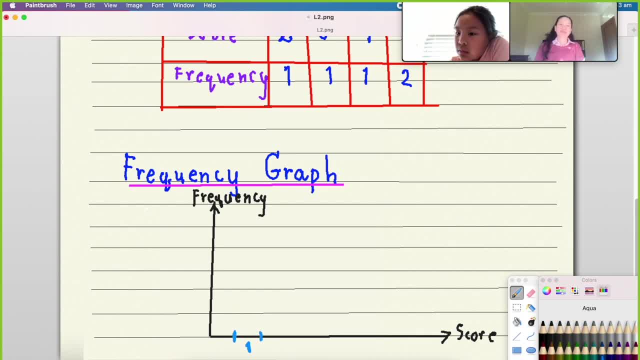 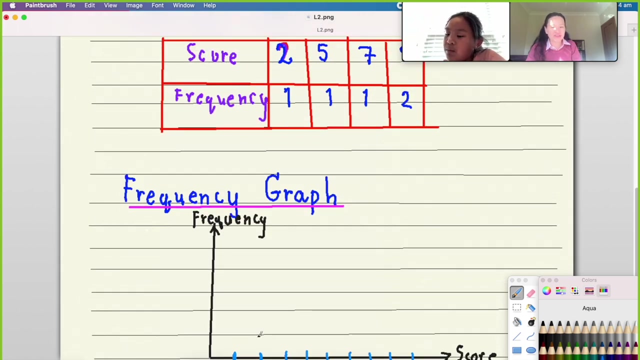 write down between that small line, like write down in the middle. is it make sense? huh, okay, we have two, three, four, five, six, seven, eight. okay, like this one, we have a score two. we have frequency one. how about we put in the exit y, one, two, three. 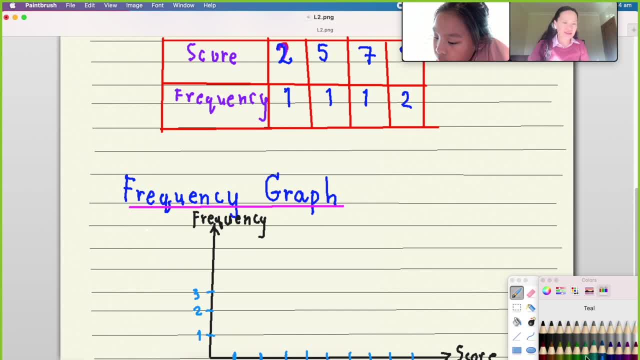 okay, we have two, three, four, five, six, seven, eight. okay, like this. one, we have a score two, we have frequency one. how about we put in the exit y: one, two, three. okay, I just put one, two, three, okay, score one. we don't have any information for.